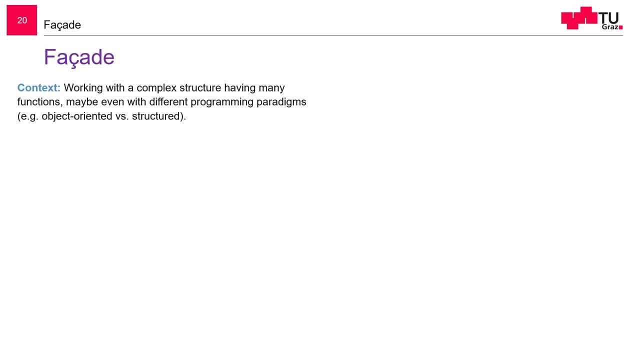 So the façade? What is the context? So we are working with a complex structure of objects and maybe objects which have different programming paradigms. For example, if we want to call some methods from so we are programming C++, so we can do object-oriented programming, and we are calling a library from C, which is a structured approach. 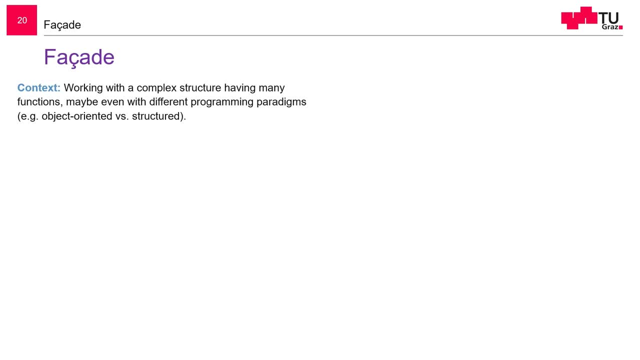 We have to use different paradigms which we are not used to. For example, legacy databases could be built up in this structured way that we always have to call some methods in order to do something, and instead we want to use an object-oriented way. 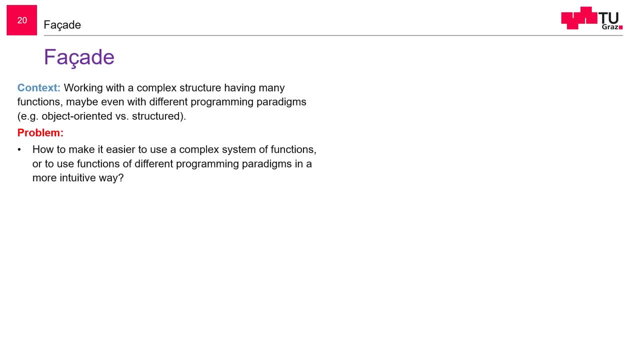 So the problem is: how can we make use of a complex system without this complexity? We want to use it in a more intuitive way. Think of the machine learning library by Google, which has just some very high-level methods to train our neural net, to test it, and so on. We do not have to cope with all the mathematics underneath. 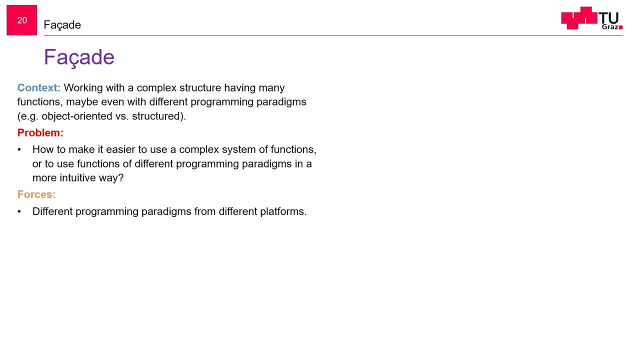 Sometimes we use different programming paradigms from different platforms and developers are used to their own environments. So if a Java programmer and a C-sharp programmer or a Java programmer and a Python programmer clash together, they fight what is the best programming language. 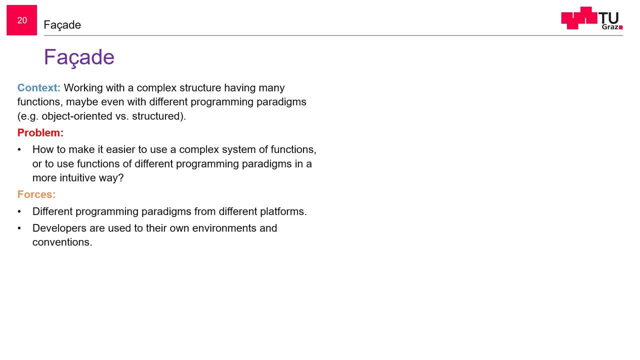 Actually there is no best programming language. But still, users are accustomed to their own environments. You always want to program in this language which you know best. If you mix up all those paradigms it becomes very difficult to maintain. That's why in the first semester of computer science in ESP, you have really to stick to this single coding standard. 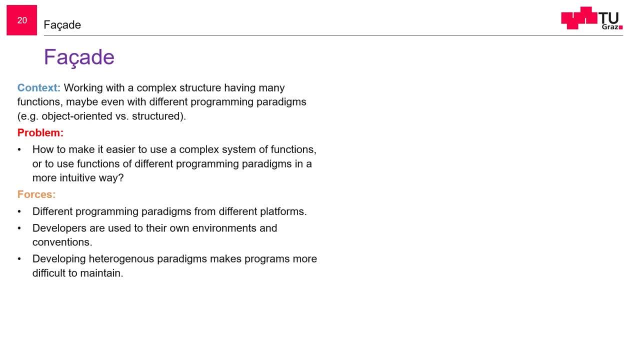 And later on. it's also very important to stick to a common standard, to a common paradigm, in order to make it readable and maintainable. Also, if you use some external library, we can not change the source code, So this is the same as in the object adapter.